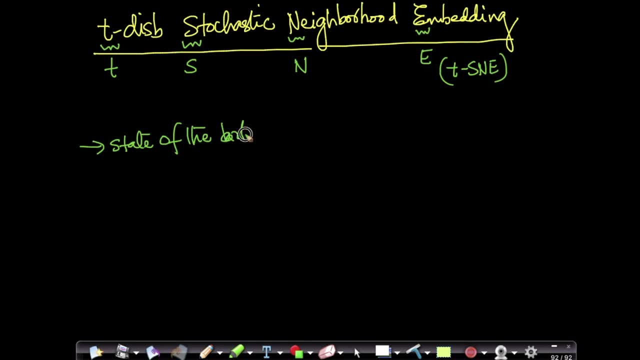 one of the best state-of-the-art or one of the best dimensional reduction techniques that we have, especially for visualization, So especially for visualization of data. this is probably one of the best techniques we have. So we did learn PCA right A while ago in the previous videos. PCA is a very, very basic, fairly old technique. right, We saw in 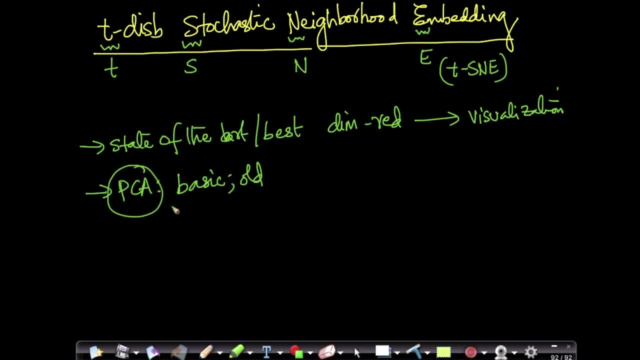 the case of MNIST, that PCA wasn't doing really good job except for zero. So we saw in the case of MNIST data, that it was not doing a very, very good job in separating out all the digits when I was trying to do a two-dimensional visualization right. So I took V1 and V2 and I showed you a. 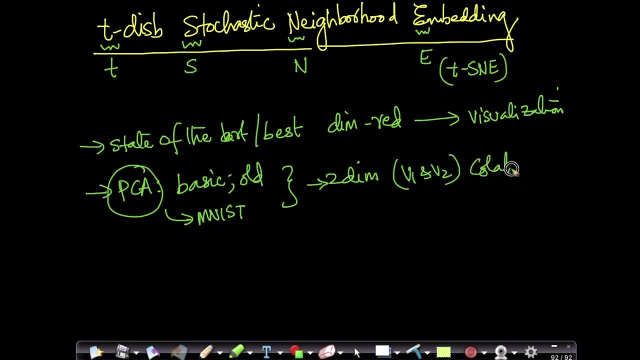 two-dimensional visualization in Christopher Ola's blog, right? So while PCA is, PCA has its own applications. there are lots of techniques. so you might say, why are we learning t-SNE, right? What about other techniques? PCA- you're calling it very simple and you're saying: 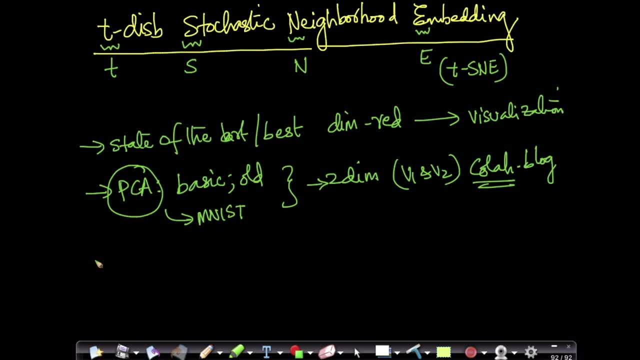 t-SNE is one of the state-of-the-art, one of the best. Are there other techniques in between? Yes, there are techniques like multi-dimensional scaling, salmon mapping, and there are also graph-based techniques, which all these techniques have been developed over the last 20 or so years, almost the last 20 years. While these techniques 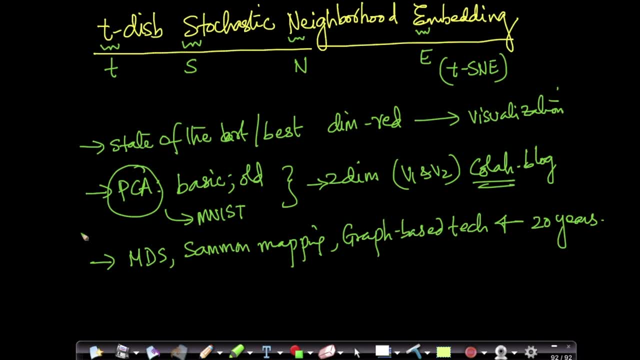 are very important. we said it's important because in this course we are trying to cover the techniques which are most used in the industry, right? So that's why we chose to cover PCA and t-SNE. By the way, t-SNE is a very, very young technique. it was the actual paper for t-SNE was published. 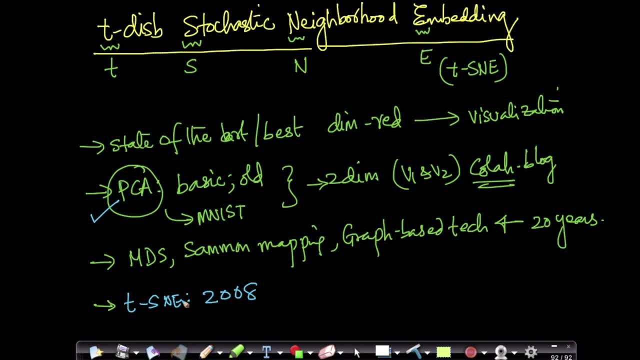 in 2008 by by a phenomenal group of researchers called Lawrence and Jeffrey. Jeffrey Hinton is, by the way, the godfather of modern deep learning- a phenomenal researcher. Anyway, we'll learn more about Jeffrey Hinton's contributions when we learn deep, deep networks. 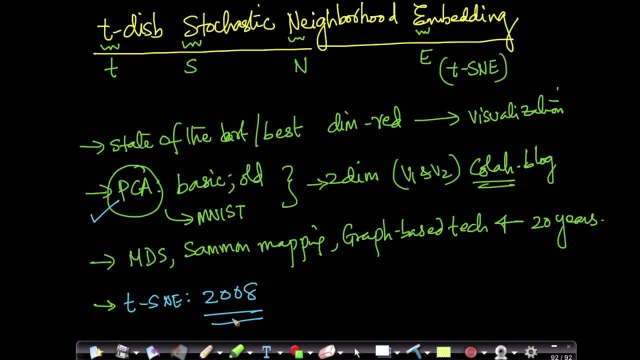 and when we learn about neural networks and deep learning. Okay, so this is this is this is like today. we are in 2017, so this is slightly under 10 years old technique and it's- it's really, really state-of-the-art. The mathematics behind it are also fairly advanced. Now, as far as t-SNE is, 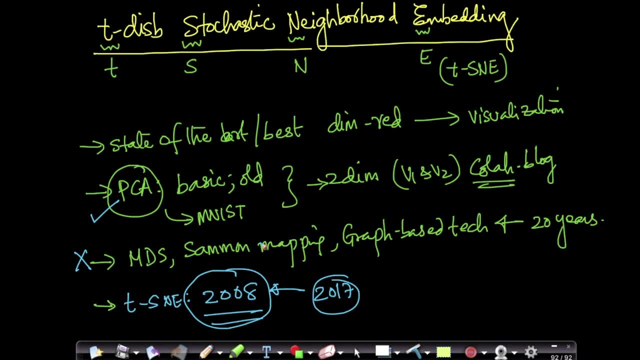 concerned. this is a very, very advanced technique. It's a very, very advanced technique. It's a very state-of-the-art. So we we are not covering MDS, salmon mapping, graph based techniques, etc. because we believe that t-SNE can do better than most of these techniques. in most cases, I'm not. 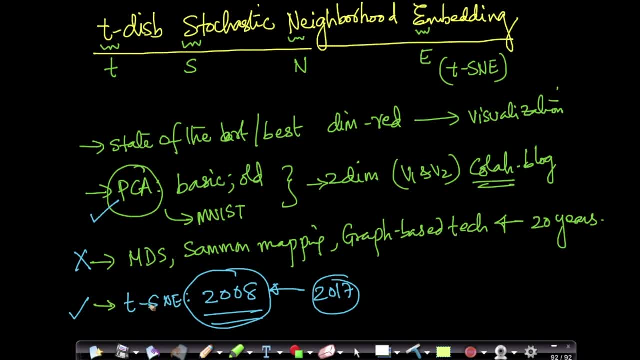 saying: these techniques don't have applications, but t-SNE will do a pretty good job or very, very comparable job to other techniques and hence we are covering PCA and t-SNE in our dimensional reduction sections. Now you might ask: okay, what is the? what is so special about t-SNE? 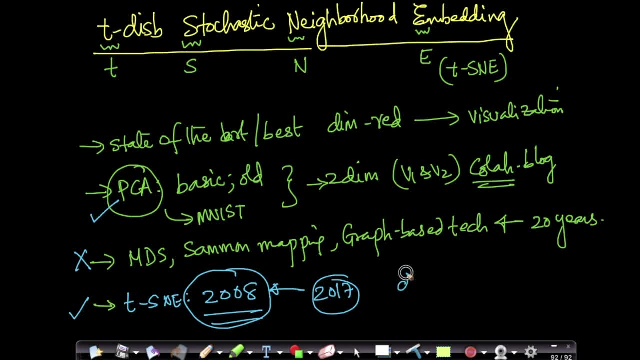 By the way, t-SNE works very well for visualization, which means if you're given d-dimensional data, I can map this to 2d or 3d data. okay, using t-SNE and the visualizations that I get from the visualization that I get after t-SNE in 2d are terrific. they're really. 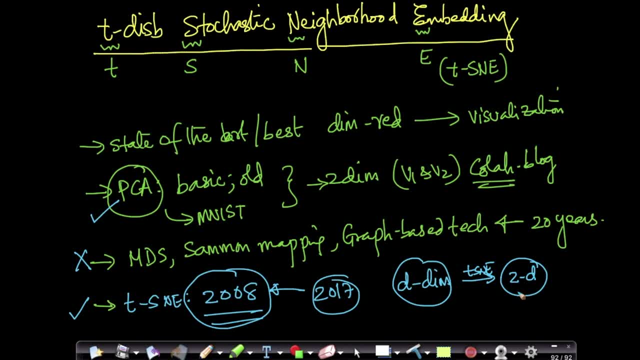 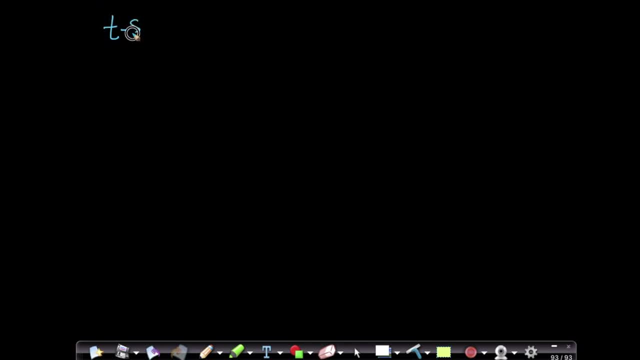 really beautiful, really really clean and very easy to understand what's happening. Now you might ask: how is t-SNE very different? at a very, very intuitive level, What is, what is the fundamental difference between t-SNE and PCA? Of course, we'll understand it much better when we learn the 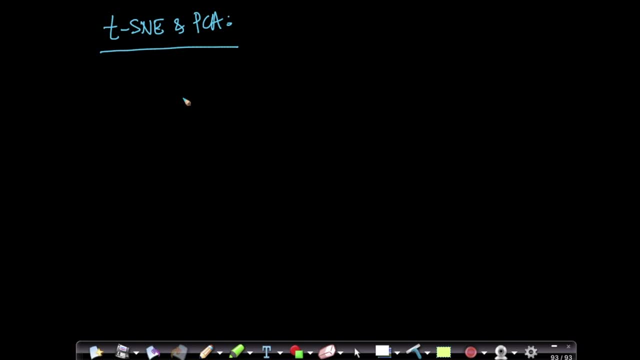 internals of t of t-SNE. but let me give you a one, one key point here. imagine if, if I have a data set like this, right, we saw this data set when we realized that when we really this is one type of data set where, okay, suppose, if I have a data set like this, okay, it says you might have a data. 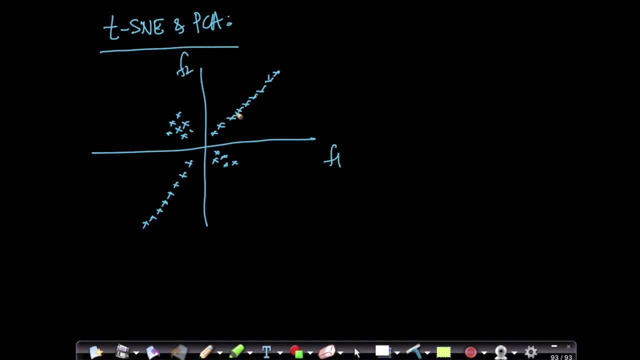 set like this: this is feature 1 and feature 2. what? what is my, my, my key, my v1 will be in this data set direction if i'm trying to project data from 2d to 1d. right, this is a cluster of points. this is a 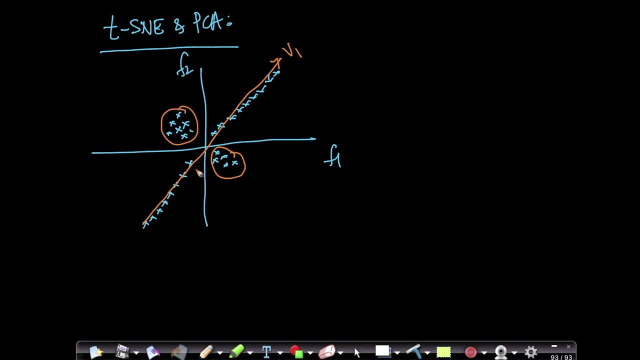 cluster of points. right, so what happened? so we saw this as one of the limitations of pca, right? so what happens? when i try to, when i try to project all the data to v1, these two sets of points will now get projected onto a small on the same area and we lose the information that